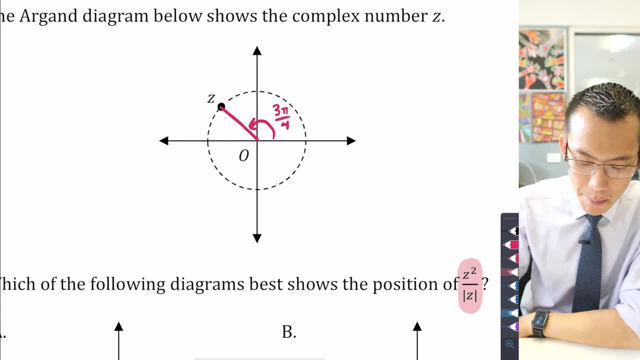 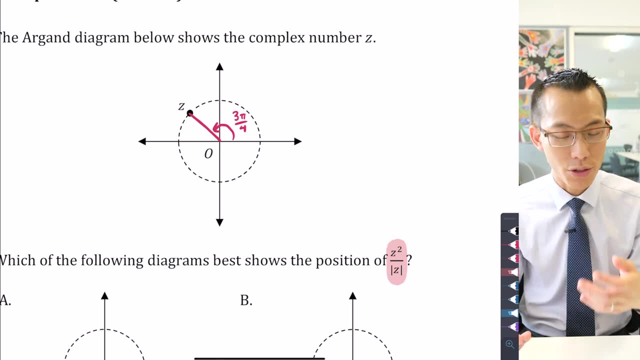 that's three quarters of pi. Now, when you are multiplying a complex number by itself, what happens is because you're adding arguments and multiplying moduli. what happens is you are going to get further or closer away, depending on how far you need to rotate around. So if you're 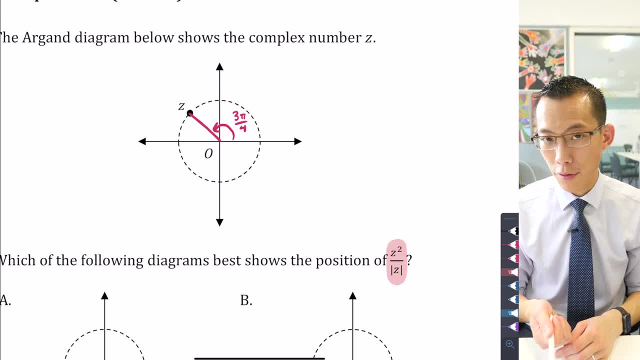 going to get further or closer away, depending on what the radius of that circle is. but more importantly, for our purposes, here you're going to rotate and because you've got an argument here of three pi on four, we know that we're going to add those arguments together. so you get three pi on four. 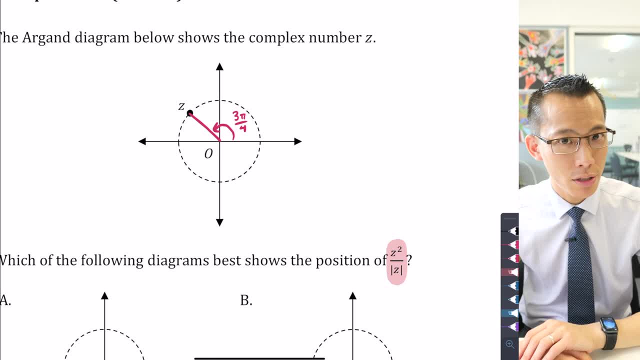 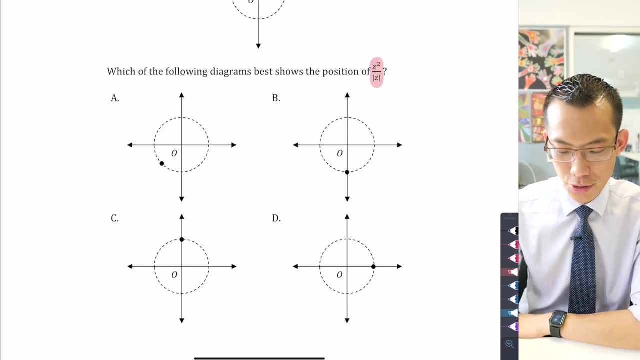 plus three pi on four, which is going to be three pi on two. It's not a principal argument, but I don't need it to be a principal argument to be able to tell a, b, c and d which is the most plausible option. You can see down here, b is going to be the best option because the argument to b, you can see. 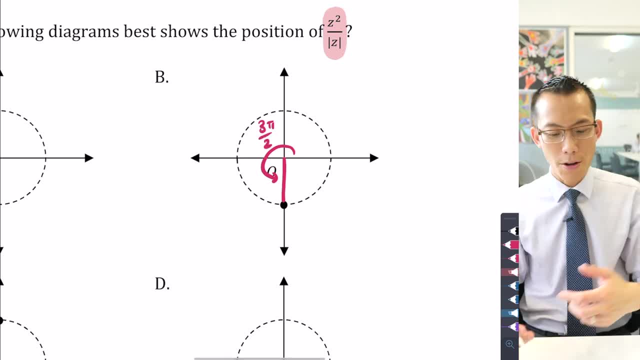 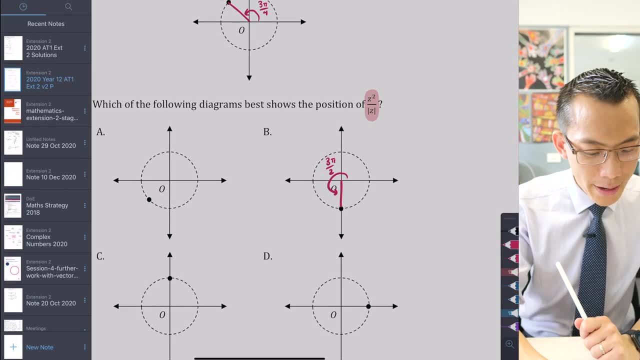 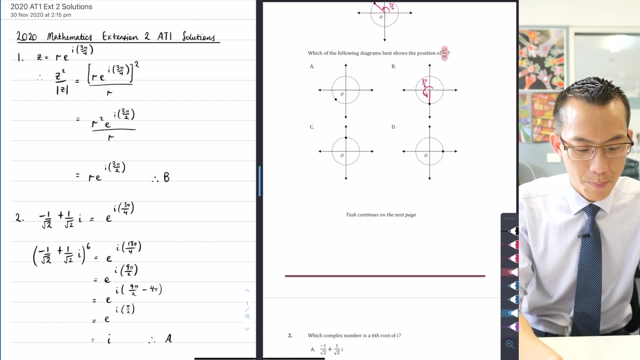 on two rotating around like so. So clearly, even without going any further into a, b, c and d, as the different options, b is clearly the best one I will point out. if you want to do this again in a more sort of algebraic way, I can just define z to be some complex number with an unknown modulus. 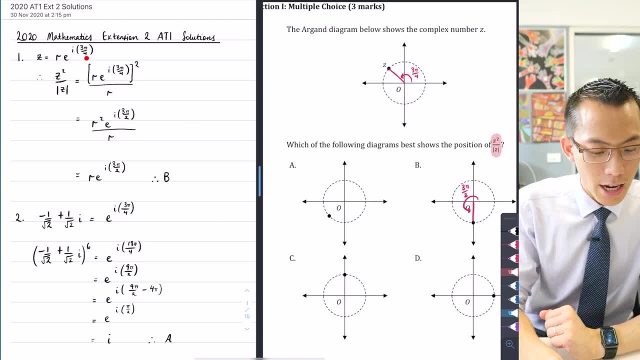 because, remember, I don't know how big this circle is, but I know that the argument has to be about three pi on four, because you can see where it sits on the complex plane. So when I go through and I square it, this is what I get on the numerator, the modulus of z, if we use this re to the i theta. 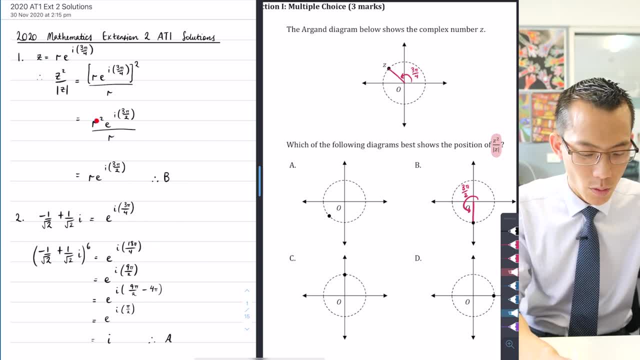 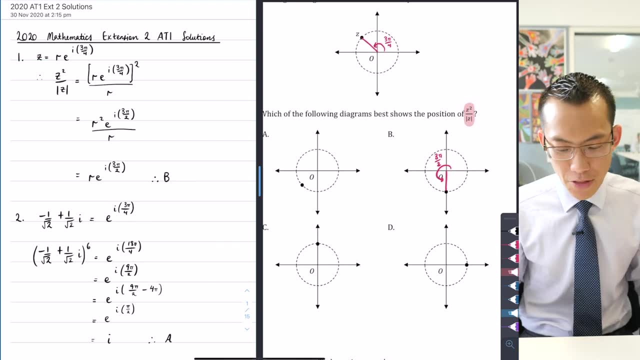 notation, the modulus of z is just r, So you can see. that's why I'm dividing through. r squared by r leaves me with one r if you come back to the diagram. that's why your options a, b, c and d- they're all on the circumference of that original circle and that three pi on two I got from. 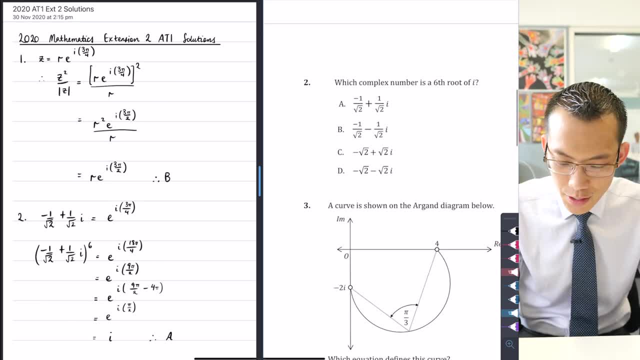 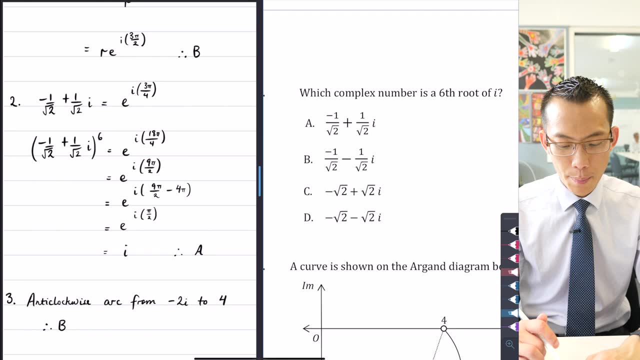 doubling this angle over here. All right, so then question two: which complex number is a sixth root of i? Now you can see over here, I've gotten an answer of a six root of i and I've got a six root of a. but before you get to that answer, you can actually very rapidly exclude some of the answers. 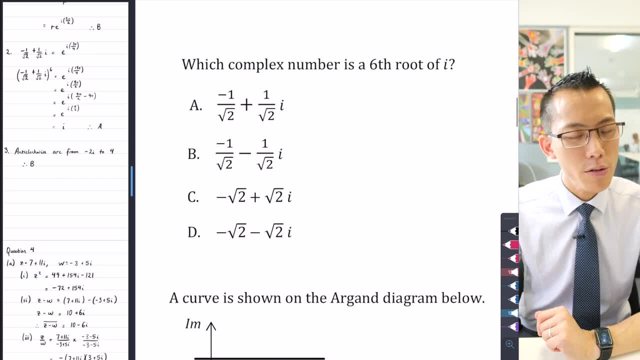 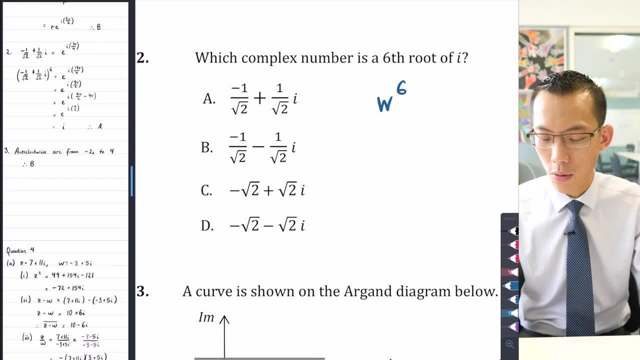 that are nonsensical. For instance, the sixth root of i right, so this is some number. let's call it, say, w, and when I raise it to the sixth power, I should get i. Now, as we noted before, when you multiply complex numbers by each other, there's going to be rotation, but there's also going to 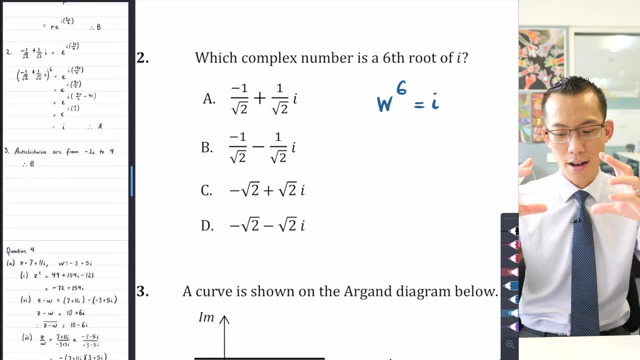 be scaling right Now. if you have a number that is further away from the origin, then as you multiply, it scales up further and further and further. and so, since I know that i is actually on the unit circle, that tells me that these two options here, c and d, are immediately irrelevant because, you know, 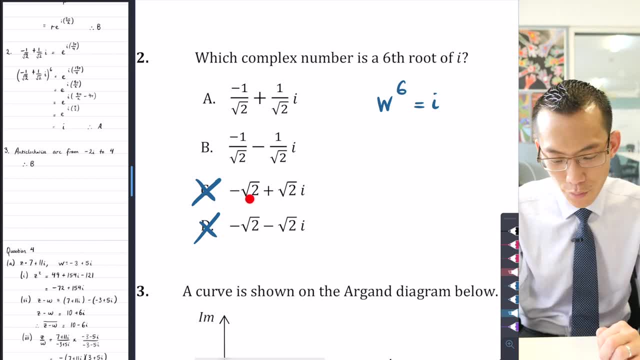 root two is about 1.4. so this is negative 1.4 plus 1.4i. so where would that be on an argand diagram if I were to draw a very rough argand diagram here and put- let's put a unit circle on here, because 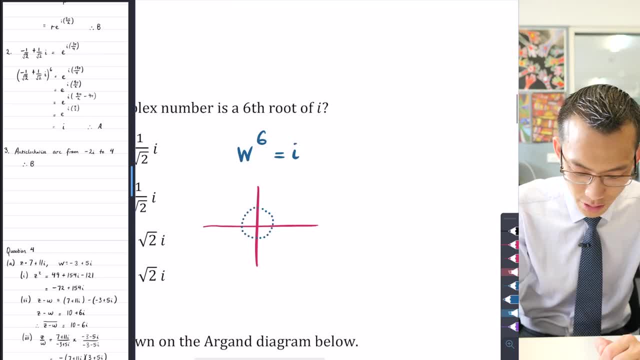 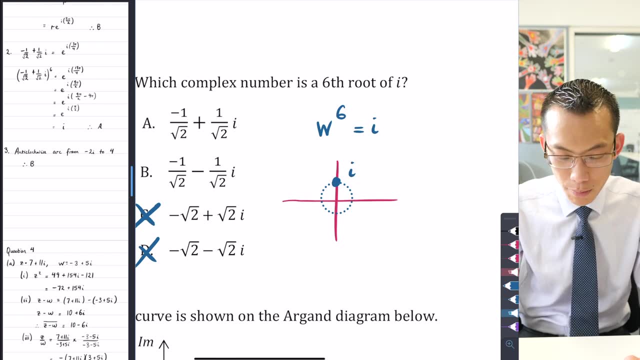 that's an ellipse. that's not what I wanted. let's draw something a little more circular so it recognizes that's better. so if we place i here, where would negative 1.4 plus 1.4i? where would that sit? 1.4 is about that far and that far, so I'm guessing it'll be somewhere up here. now it's. 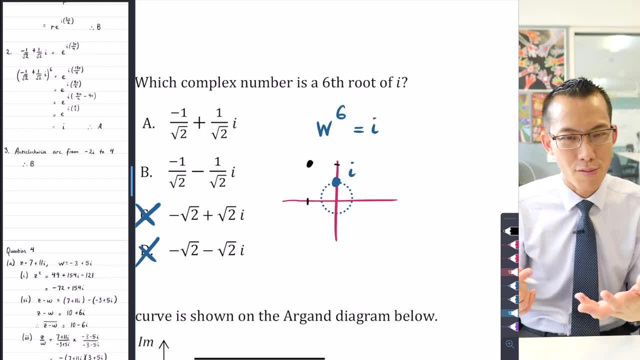 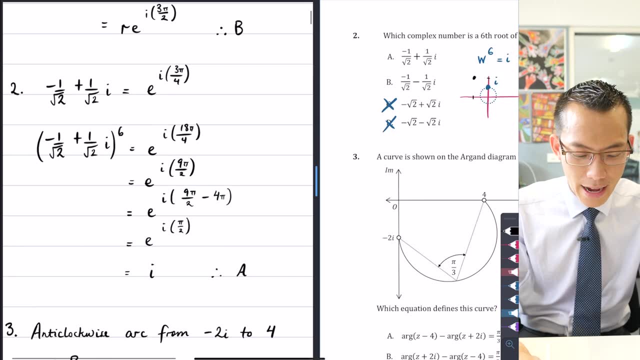 clearly too far away. when you multiply that, even by itself, once right, you're already away from the unit circle. you're just going to get further and further away. so that's why I've eliminated options c and d, and then to work out out of options a and b which one is better. again I think about 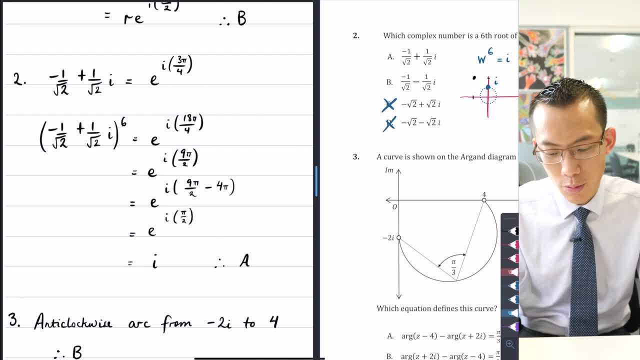 the arguments. that's the key difference between them. minus 1 on root 2 plus 1 on root 2i has the same modulus as minus 1 on root 2, minus 1 on root 2i, because they just sit in different quadrants. 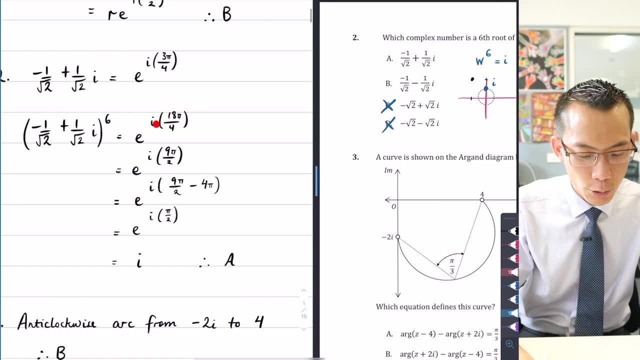 so that's why you can see over here I'm really focusing on the angle 3 pi and 4. if you raise it to the sixth power, you're just multiplying that index by 6, so 18 pi and 4 becomes 9 pi on 2. 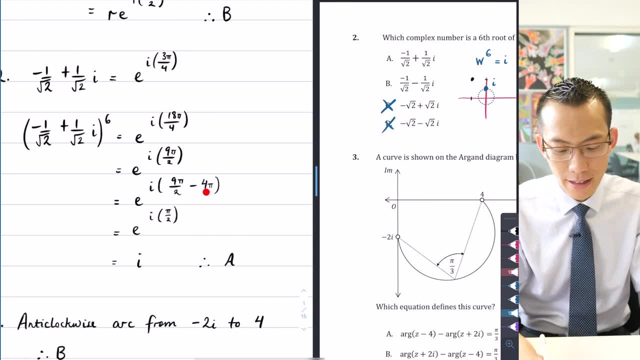 9. pi on 2 is an enormous argument. so I'm subtracting integer multiples of 2 pi, because that's full revolution. so this is two full revolutions. that brings you back to pi on 2. that's i, which is what I wanted after all. so 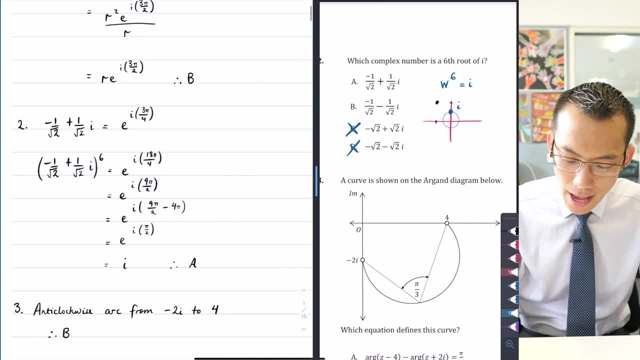 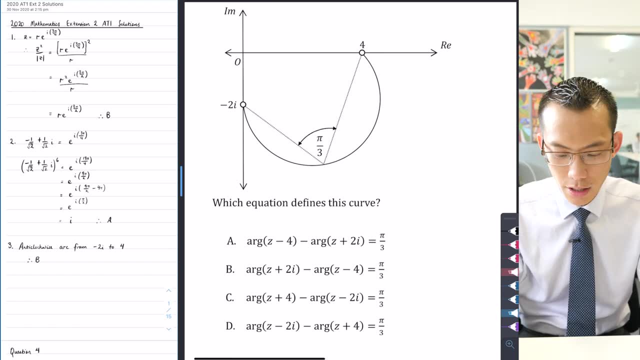 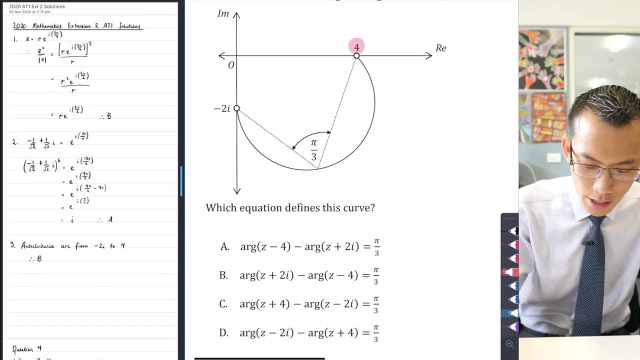 that's how I know. the answer is a. and then here comes the last multiple choice question. so here's this curve on the argon diagram. below which equation defines this curve? well, we know it's going to between be between this point over here, 4 and this point over here, minus 2i. so therefore, 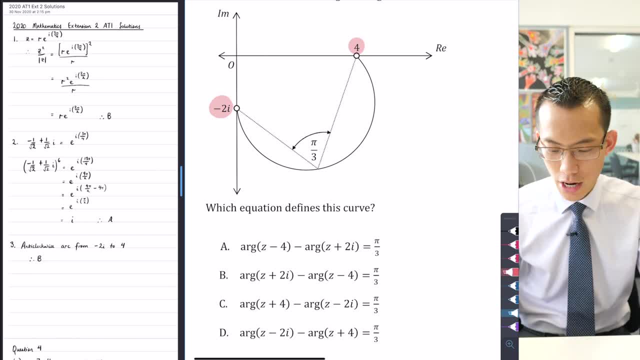 remembering the form of all different minor and major arcs. we need something that's of the form: stay on red. I guess z-4 and also this is z-2i, so that would be z plus 2i. so when you have a look you can see again. I can remove some options fairly quickly because you've 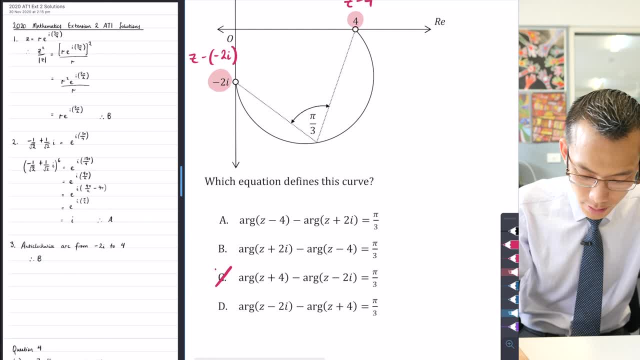 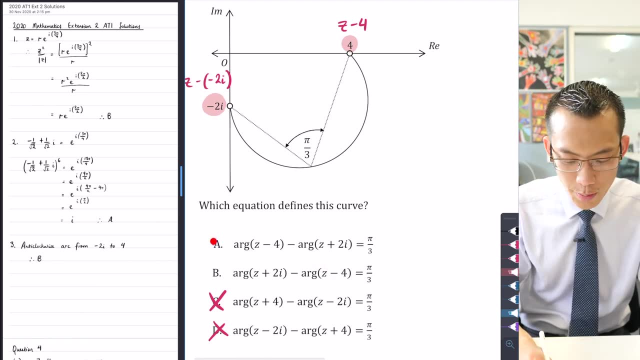 got these z-2i options over here, c and d, and then you can see, oh, z-4. well, this is the case in both of them. so now I have to choose between a and b. what's the difference between a and b? well, you've. 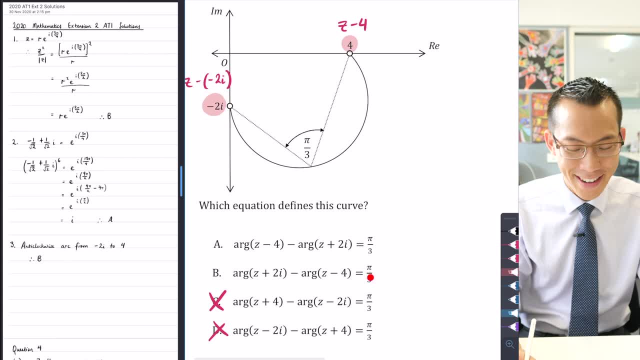 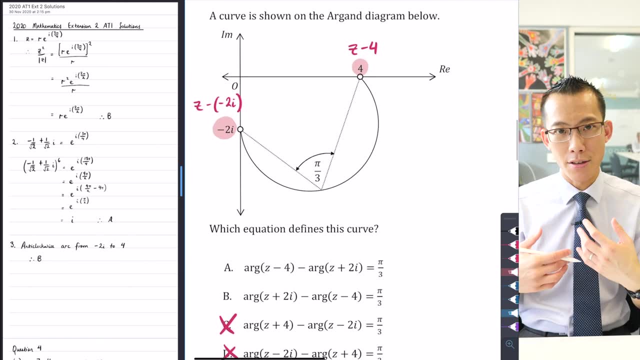 4 is the same, the z plus 2i is the same, the pi over 3 is the same for all of them. The difference is where's your start point, where's your end point. So you can see. I need to count or measure my angles anti-clockwise, from a start point. 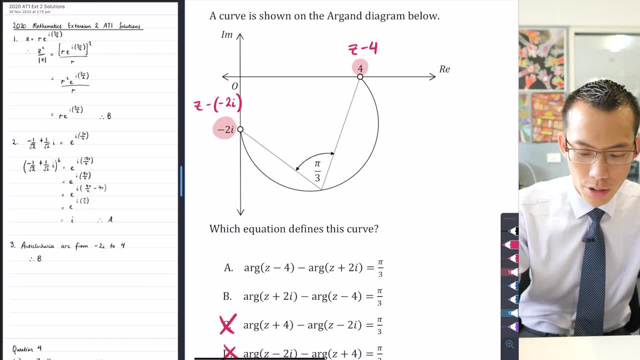 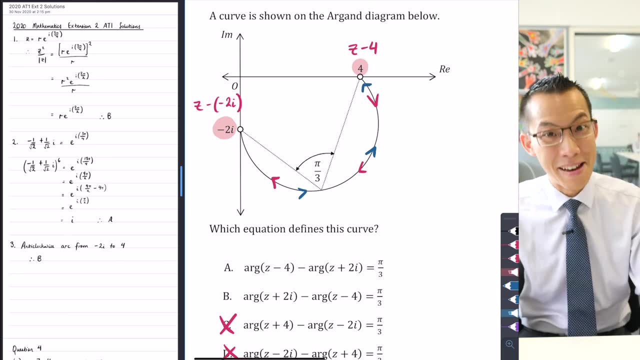 to an end point. So is it anti-clockwise to go in this direction, or is it anti-clockwise to go in this direction? And if you think carefully about the direction that a clock goes in, it's clearly going to be the blue direction, right? 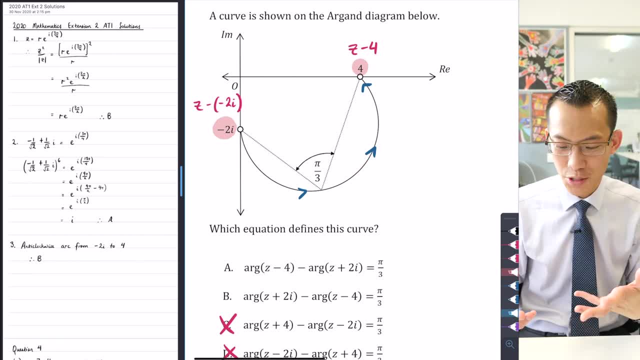 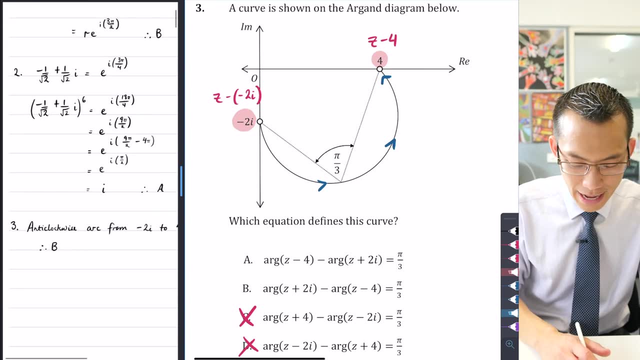 So, therefore, get rid of these red arrows. So I have to start from minus 2i, then I've got to go to 4, and that's why you can see I've written anti-clockwise from negative 2i to 4, and that's option B. 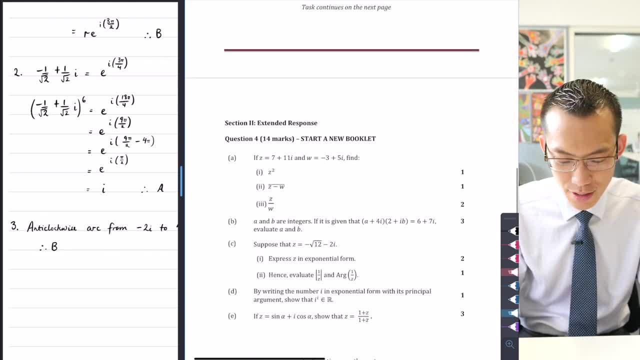 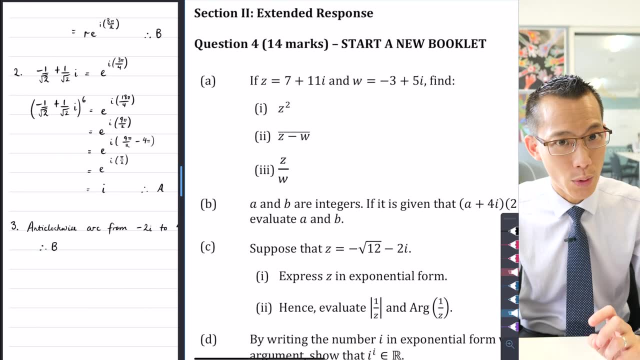 So that's all the multiple choice questions. let's now dive into the extended response. 4a starts with some warm-up stuff here, to be honest, just some simple, straightforward, complex number arithmetic. So we define for you a particular z and a particular w. 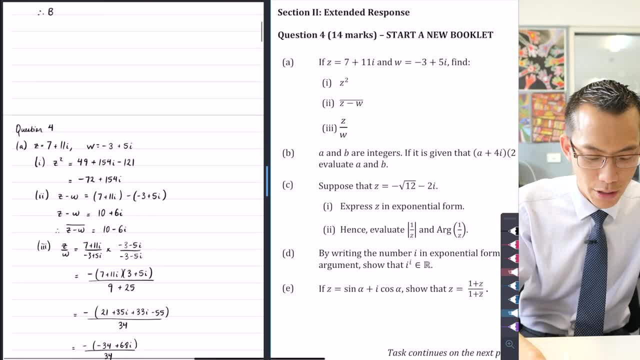 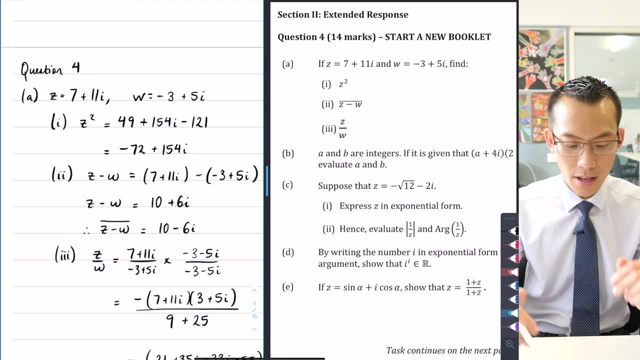 How do we square it? Well, I won't go into too much detail in this one because I think you'll be okay handling it. You can see, all I've done here is this is just 7 plus 11i, and I've just expanded the. 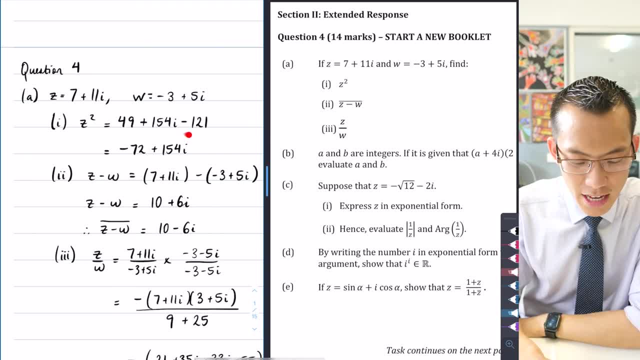 brackets when I square it. So there's my 7 squared, there's my 11i squared, noting that the i squared has become a negative 1, and this is double the product of these two. So 77i is the product of these two. you double that, you get 154i. 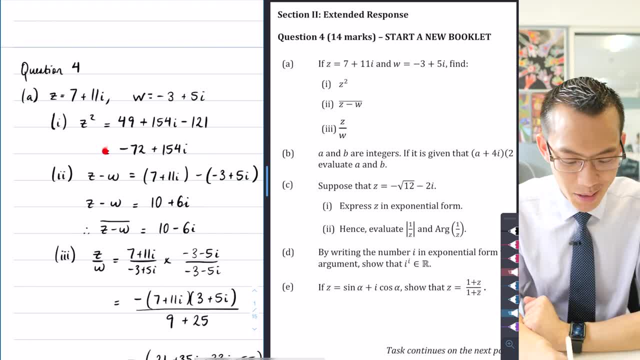 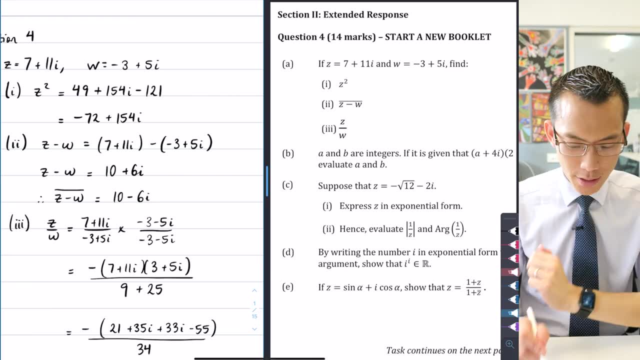 Don't forget that Your complex numbers do have imaginary parts. So this is what you get for z squared. When you have a look at part two, you can see in my working I've done this kind of in two parts. Firstly I've said, oh, you want z take away w. so that's what I started working out over. 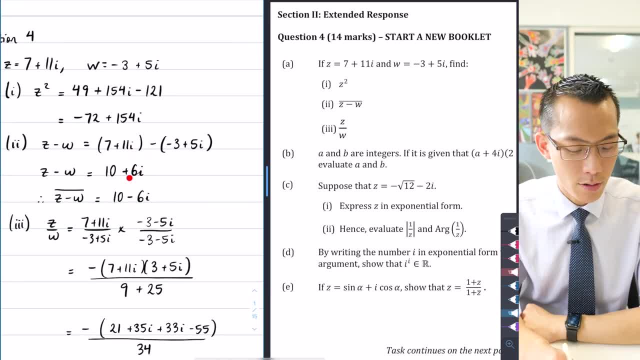 here. So this is just my straight substitution. and then I've collected like terms, real and imaginary parts. But then secondly I noticed the question is also asking for the conjugate of z minus w. So that's me taking the imaginary part and just flipping the sign. 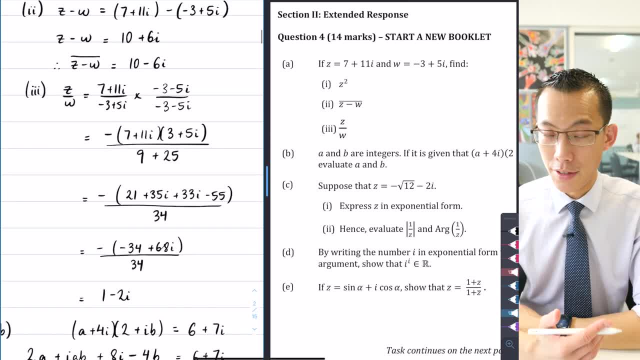 So that's part two. And then, lastly, for part three. you can see, here is my division. So there's z, there's w, and what I've multiplied through by is the conjugate of w, because that gives me this completing- sorry, not completing- this difference of squares. 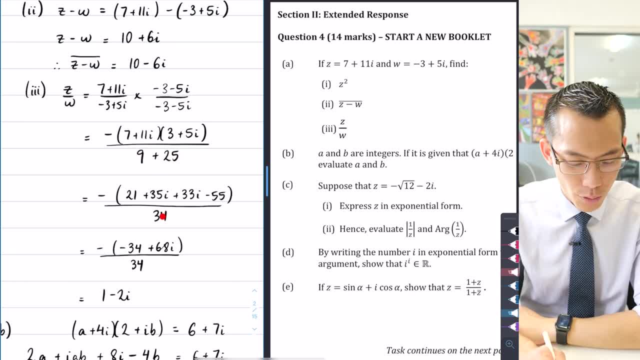 down the bottom. That's just going to be completely real. So you get this 34 down there and that eventually cancels out with what, neatly, you have on the numerator there, which gives you 1 minus 2i as a final solution. 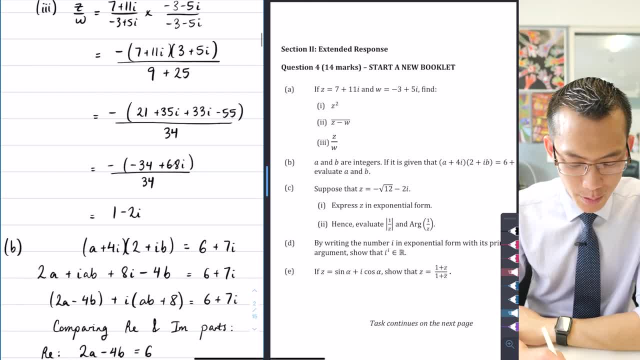 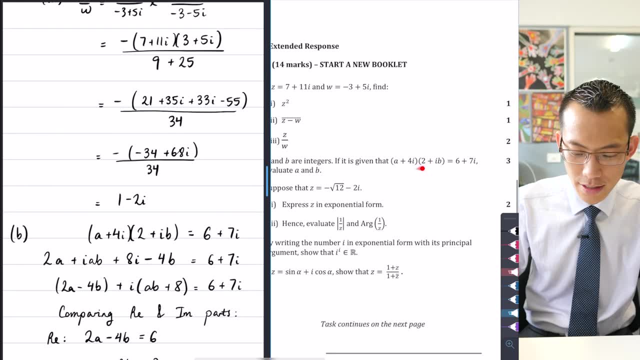 Okay, part B. Now you have to be careful with this one, right? Because I think most of us were okay to just start off. as you can see, Here's my answer here, So you can see here that you're multiplying out on the left-hand side. 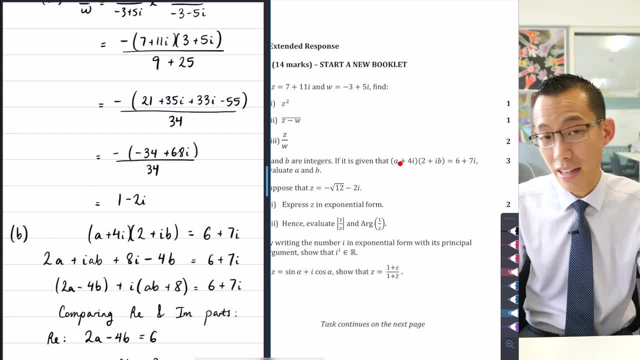 You're expanding these brackets and you're then saying, oh well, once I expand it, I'll get some real bits, I'll get some imaginary bits, and then I'm going to equate them with what I have over here on the right-hand side. 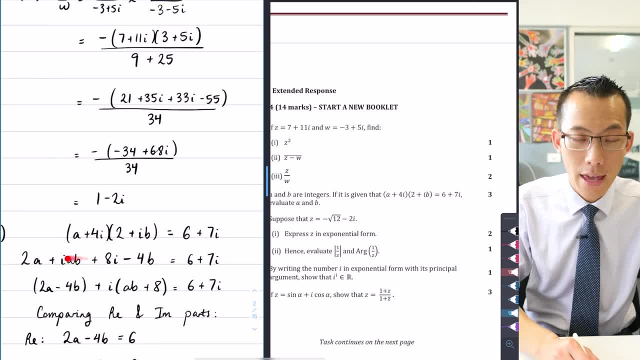 So you can see, I've already done that here in my working. Here's the first line of expansion, And then what I've done is I have said this is real and this is real, So I've collected them over here, And then this term, or this pair of terms, rather, is imaginary. 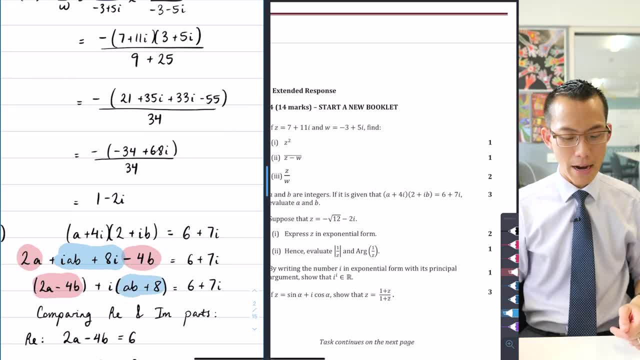 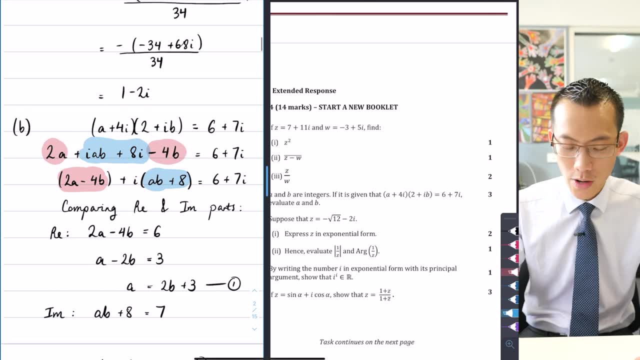 So I've factorized out the i And there's my imaginary part there. So red part's going to be 6,, blue part's going to be 7, so you'd get that And you've got a pair of simultaneous equations which you can then solve like you have solved. 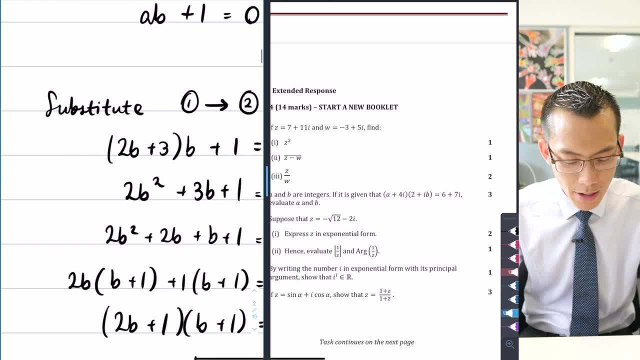 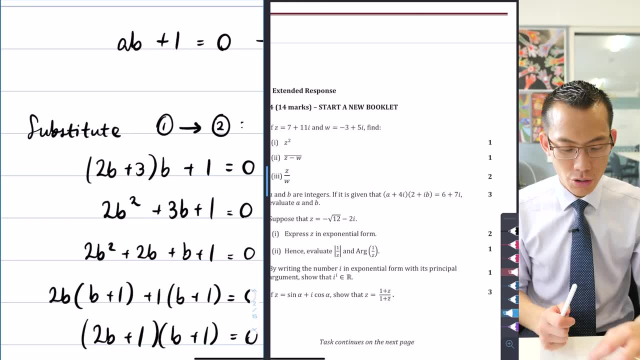 many simultaneous equations in the past, And then you get to this point. Maybe you solved for a instead of for b, It doesn't really matter, You can go in either order. But whichever order you go in, you should notice that when you get to this factorization,